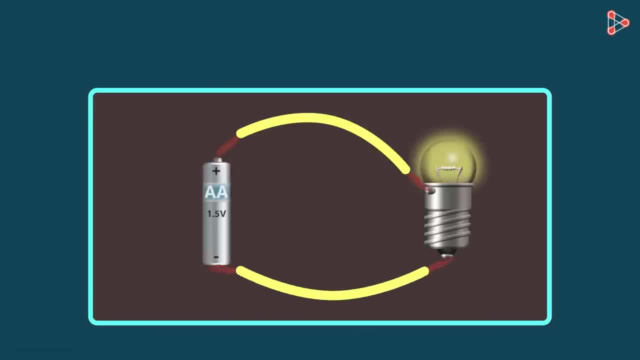 terminal of the cell to the second terminal of the bulb. The bulb then glows. The word circuit is very important here. In this context it will be electric circuit. In simple words, it is the path along which an electric current can flow. You can see. 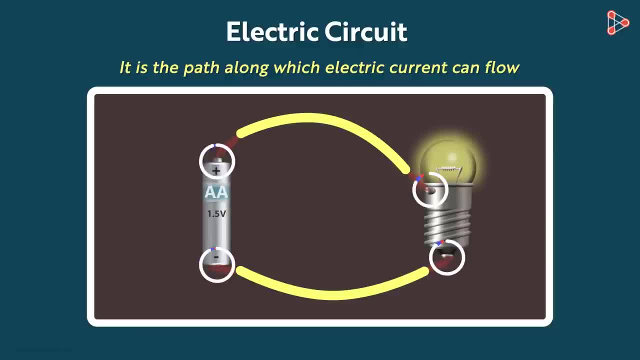 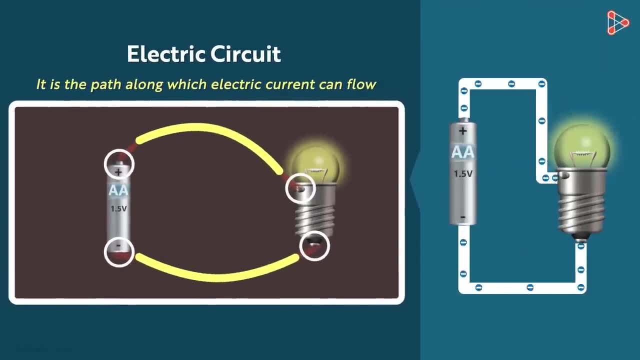 here that a closed loop is formed. All the terminals of the electric cell and the bulb are occupied, So here the electric current is flowing along a closed path. We say that electric circuit is complete, But how exactly does electricity flow through the circuit? 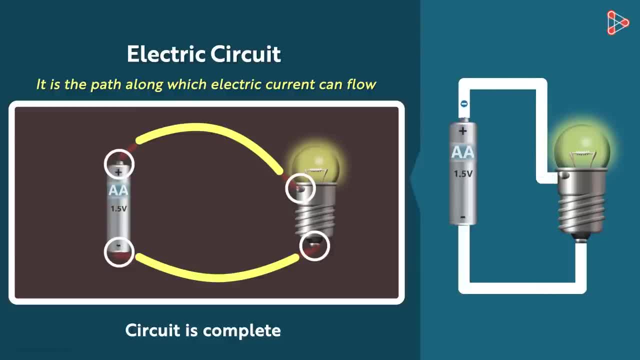 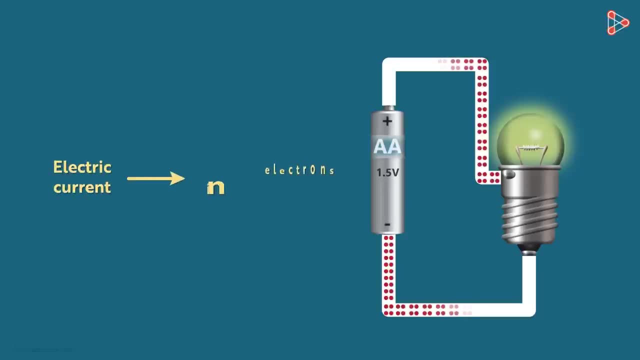 Well, it is difficult to explain how exactly it flows. However, I will try to give you an intuitive explanation of this phenomenon. You will learn more details in your higher grades. Basically, it is said that electricity or electric current is a flow of electrons. 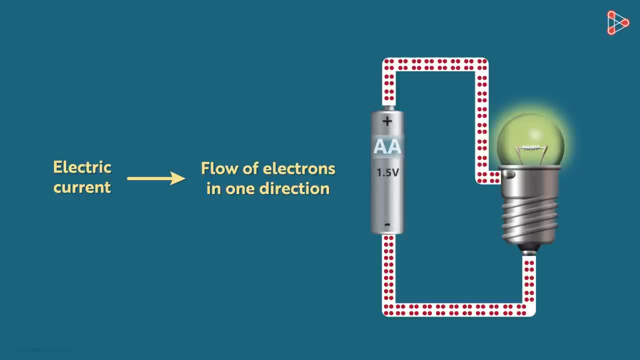 in one direction. What really happens is that the negative terminal of the cell repels the electrons in the copper wire near it, So the electrons in a copper wire are not connected to the terminal. The electrons in the copper wire drift away from the terminal, But in 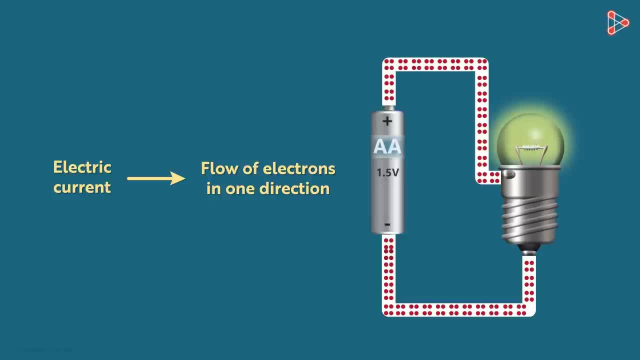 the process, they repel their neighbouring electrons, Or in other words, they transfer some of the energy to their neighbouring electrons. So the neighbouring electrons are also pushed away. They in turn further transfer the energy to their neighbouring electrons. The process continues and the energy flows throughout the circuit. This flow of electrical energy. 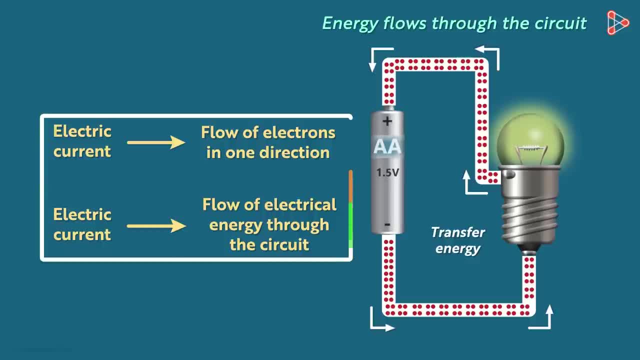 is nothing but electric current. So these are the two examples of electric current. These are the two ways to define electric current. This one is more accurate of the two. In reality, electrons don't really travel from the negative terminal all the way to. 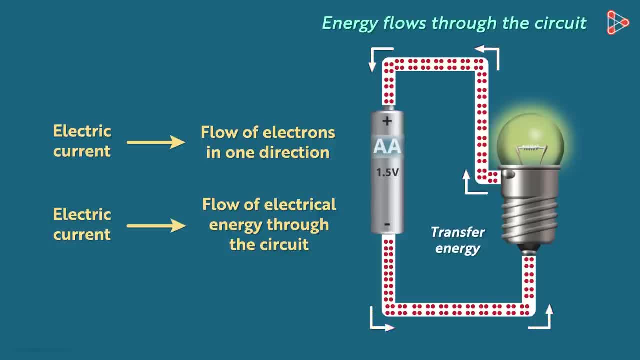 the positive terminal, The electrons merely drift slightly from their rest position and transfer the energy to their neighbours. This is because the wire is a solid object and the density of atoms per unit volume is very high. Hence, there is no space available for electrons to travel all the way to the positive terminal. 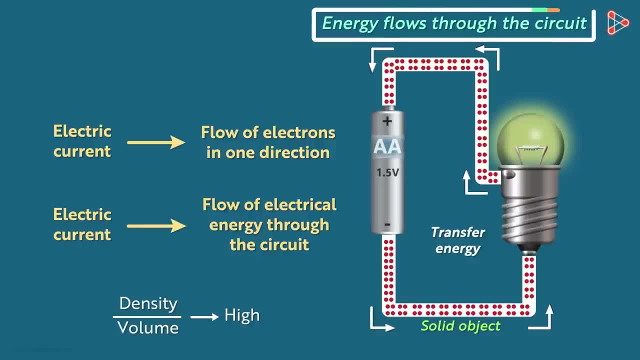 So it is this electrical energy that travels through the circuit. But how does the energy flow? through the bulb, The electrons in the copper wire transfer this energy to the electrons in metal rod connected to one of the terminals. This energy then flows through the rod, through.